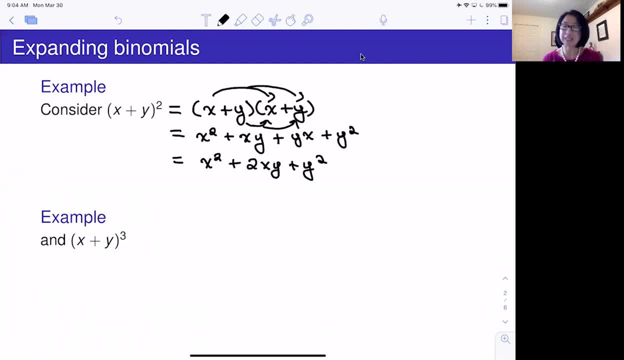 and an x from the second factor. So I don't really have any choices to make. There's only one way to do that, And that's why I only have one of the x squareds. However, when I want to try to make the term xy, I can do it by picking an x from the first factor and a y from the second. 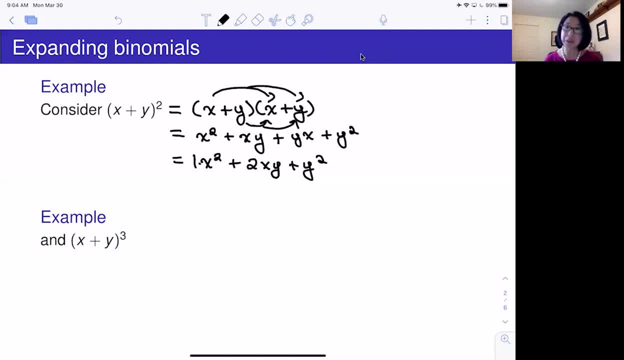 factor, or vice versa. So there are two ways of doing that. And then finally, when I want to find the y squared, I have to again pick the y from both factors, right? So then there's only one way of doing that. It's very similar. when I expand out x plus y cubed, then I get x plus y times x plus y. 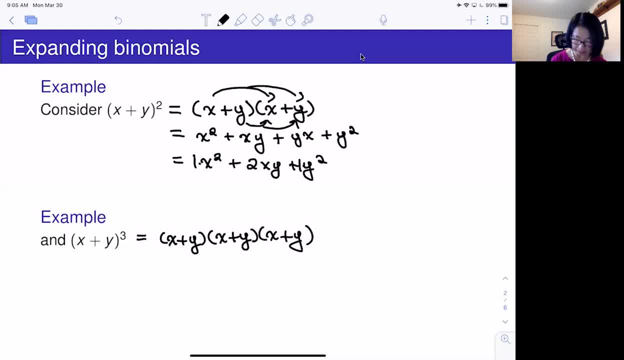 times x plus y, And we can think about what kinds of terms am I going to get? Well, I'll get x plus y, times x plus y And x cubed. And there's only one way to do that: I have to pick the vx from each of the three. 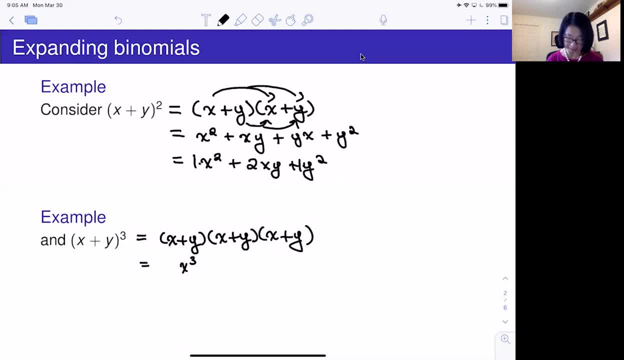 factors. So I get x cubed. And then, how many ways are there of getting x squared y? Well, let me think about this. Now I'm actually going to think about this: Instead of choosing x's, I'm going to think about choosing y's. So for the first term, I chose zero. 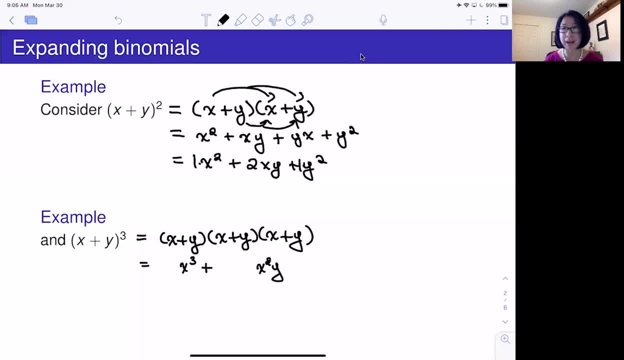 y's For this term, with x squared y, I'm going to choose exactly one, y, And that can be from any one of the three factors. So I'm going to think of this as three, choose one, And for the first time, 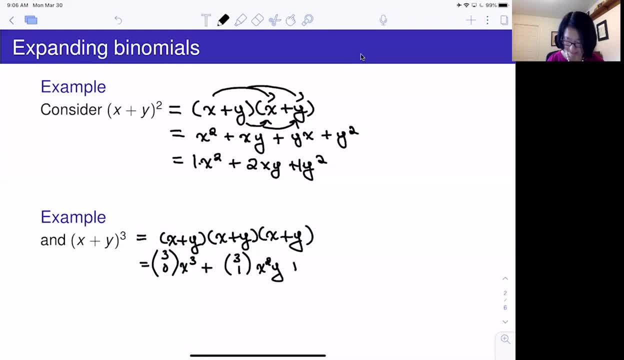 I had three factors and I chose zero y's. For the second one, I have xy squared And now I have to pick two y's from among these three factors. Oh, it's like four, Three factors, right? So it'll be three, choose two. And then, how many ways can I get a y cubed? 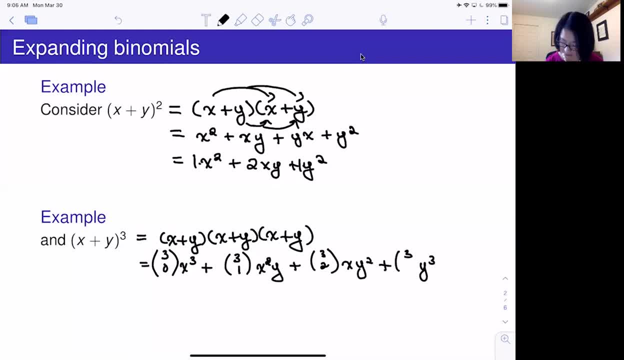 I have to pick all the y's. So I have three factors and I have to pick three y's And what you can see, if you do the careful use the distributive law carefully, is you will get x cubed plus three x squared, y plus three x. 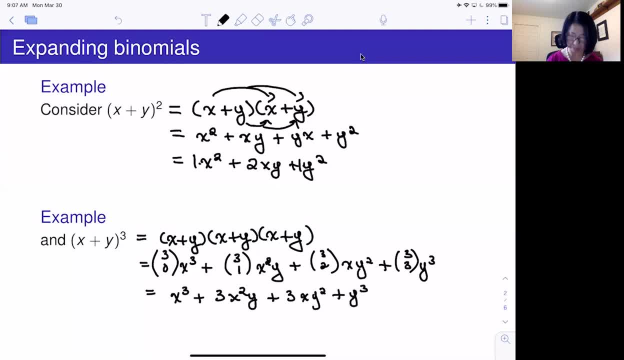 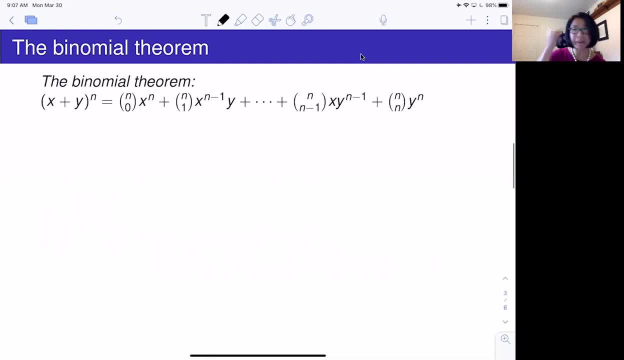 Y squared plus y cubed. Okay, All right. So those examples help us to see why the binomial theorem holds in general. In general, we have x plus y to the n is x plus y. times x plus y, where I multiply x plus y. 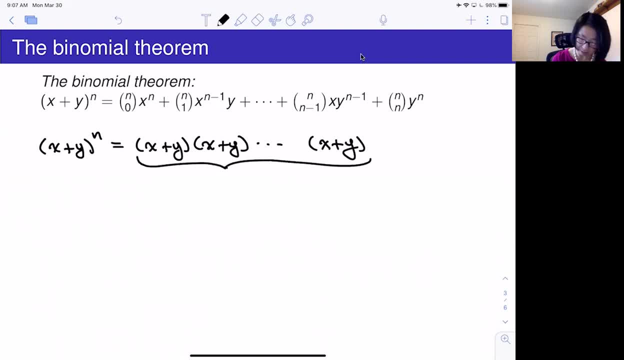 n copies of them. So these are n of them. And then I can think: well, how many ways are there to get an x to the n th? Well, I have to choose no y from any of the factors, So I have n. 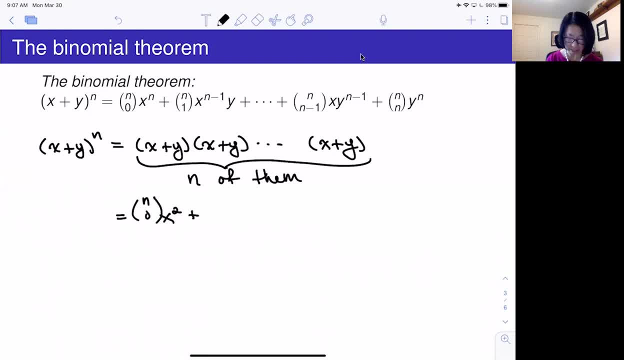 factors and I'm choosing zero y's. In how many ways can I get the term x to the n minus one times y? still have n factors. oops, I still have n factors and now I have to choose just one y from them. 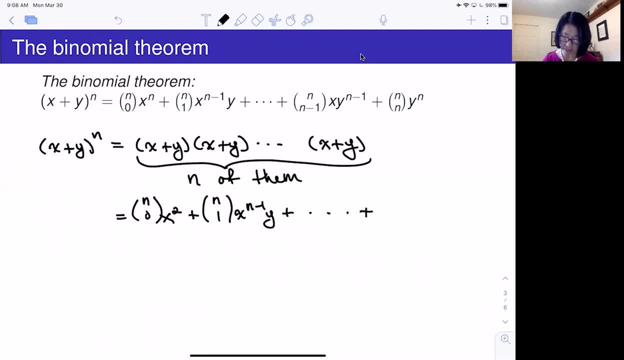 etc. Until finally, at the end, I have things like x times y to the n minus one, where I have to choose n minus one y's from my n factors. And finally, to get a term like y to the nth, I have to choose n y's from the n factors. And just remember that n choose zero. 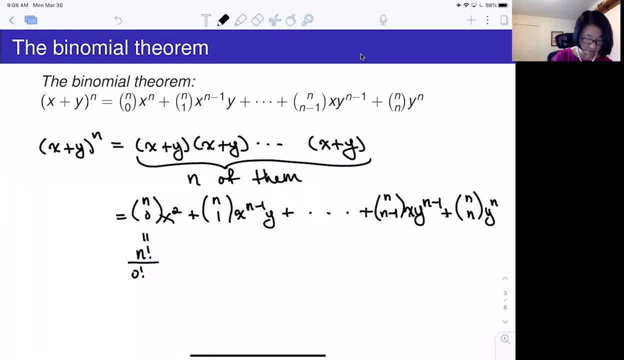 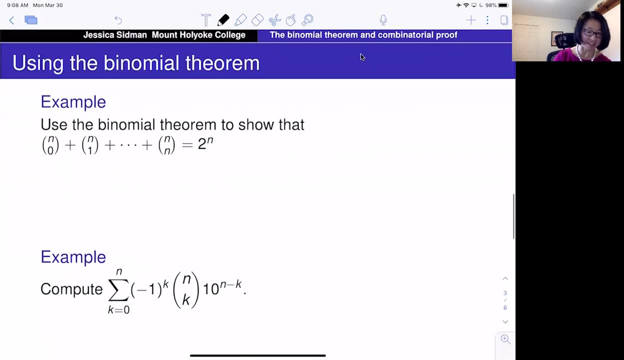 is equal to n factorial over zero factorial times, n factorial which is one, this is also one, this is n, etc. Okay, so that's the binomial theorem. Let's see how we can use it in some pretty cool ways. 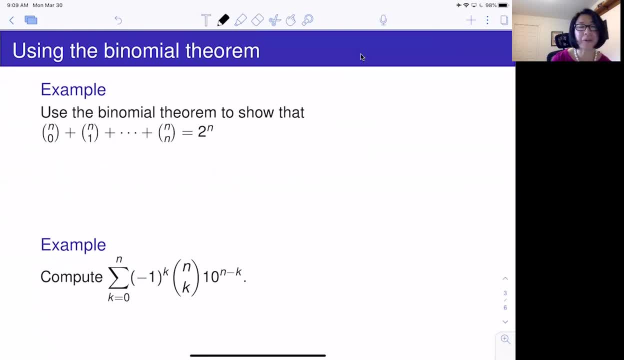 For example, suppose we have this sum, which holds for every n greater than or equal to one, that n choose zero plus n choose one through n choose n is equal to two to the n. So here's a cool way to see that it's true. So here's a binomial theorem proof. 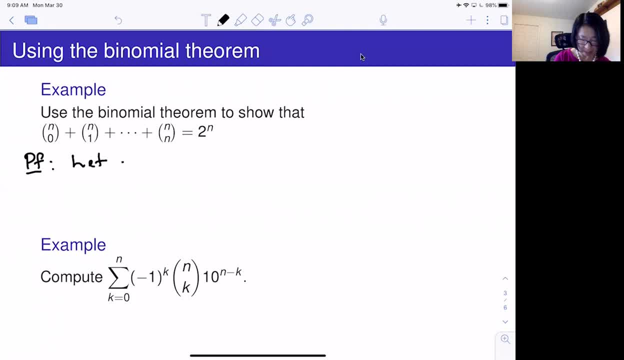 Well, what we can do is let x equal to y equal to one in the binomial theorem. So what happens then? Well, in the binomial theorem we had that x plus y to the nth is supposed to be equal to n. choose zero times x to the n plus n, choose one. 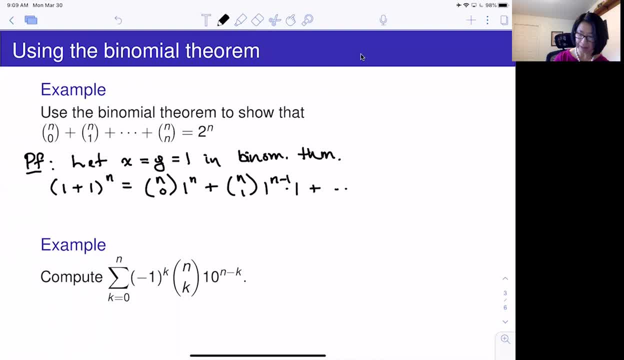 x to the n. minus 1, y plus through n. choose n minus 1. x to the oops. x to the first. y to the n. minus first plus n. choose n y to the n. but what we see is that 1 plus 1 is 2 on the left hand side and on the right hand side all those. 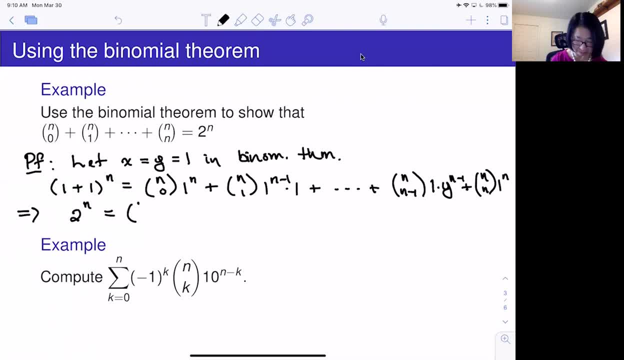 powers of 1 are just 1, so I really do have my sum: n choose 0 plus n choose 1 plus dot dot dot plus n. choose n minus 1 plus n choose n, and that's exactly what I wanted to show. I didn't have to. 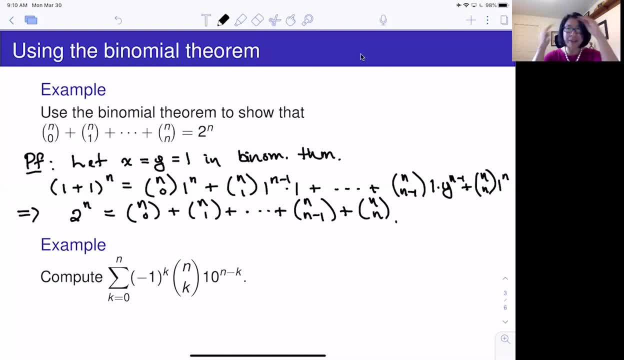 use some induction proof. I didn't have to get into that formula with the, with the factorials in it. pretty neat, huh. we can also use the binomial theorem to compute, to compute a kind of complicated sum like the one at the bottom in the example. so let's see what. 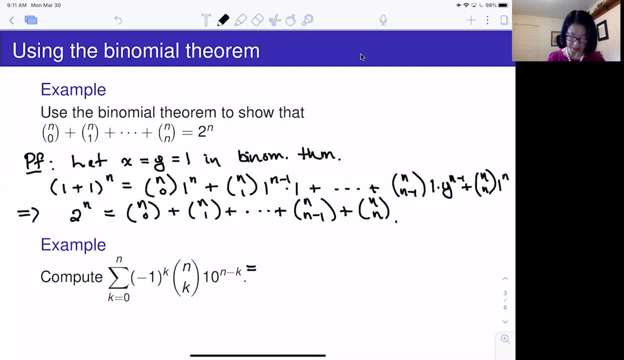 this really is. maybe we can write this out a little bit, so it's like: negative 1 to the 0 n choose 0. 10 to the n plus. negative 1 to the first n: choose 1. 10 to the n minus 1 plus. 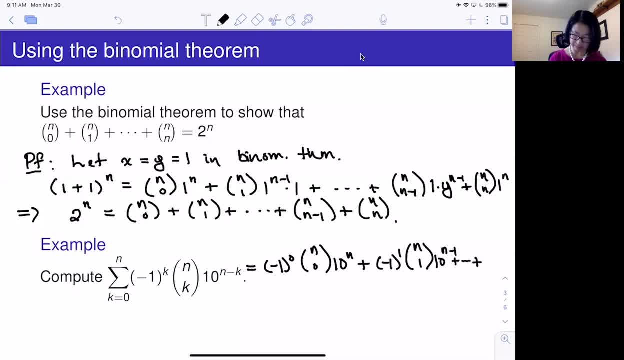 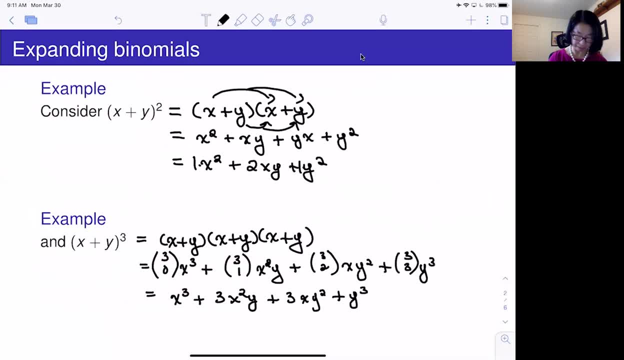 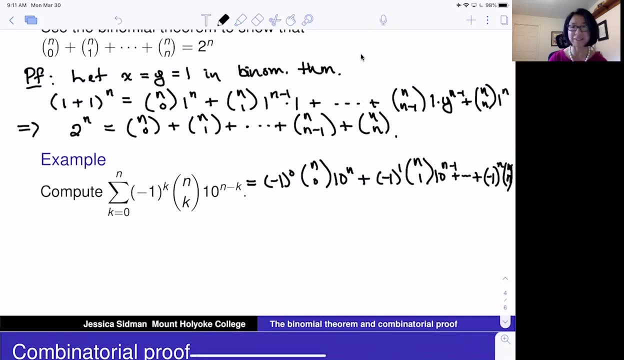 I'm gonna try to get it in here: negative 1 to the n, n, choose n. and I'm weird and it's 10 to the 0, so I'm not gonna write it, because 10 to the 0 is 1. okay, well, what is this here? let's let, if we want. 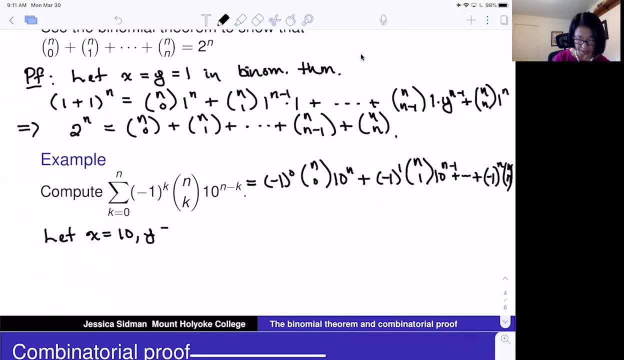 x equal 10 and y equal negative 1.. Then by the binomial theorem. so in the binomial theorem then what we have is 10 minus 1 to the nth is equal to this terrible looking sum. I'm gonna write it like this: k equals 0 to n, negative 1 to the k. n choose k 10 to the. 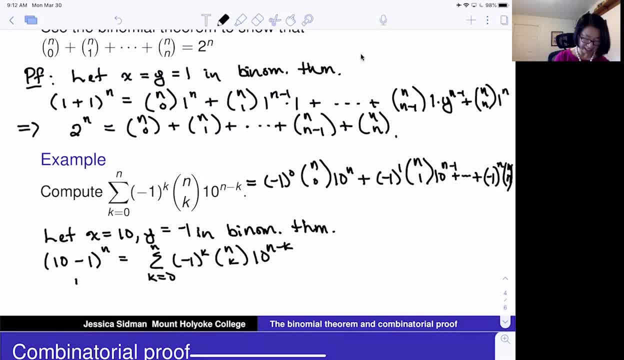 n minus k, And what we see then on the left-hand side is: this is just equal to 9, to the nth. Pretty cool, do we believe it? Like, let's do one of them, maybe, for n equals 2.. Well, let's do n equals 0.. Like when n equals 0,. 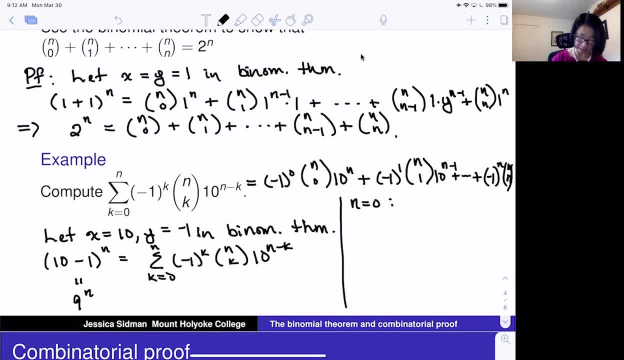 what happens? What do we get? We'll just get the negative 1 to the 0 times n choose 0, which is 0 choose 0 times 10 to the 0, that's all equal to 1, and 9 to the 0. 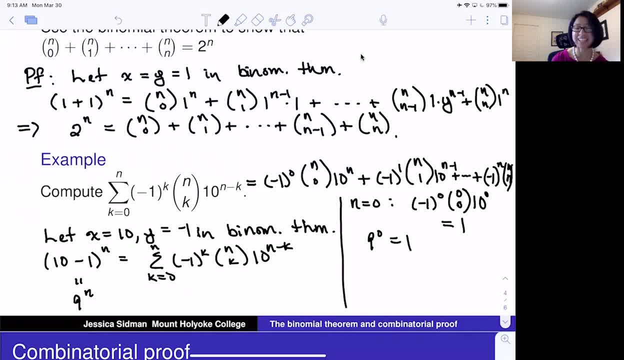 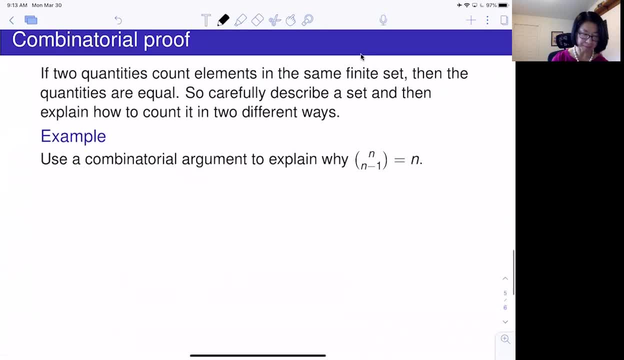 equals 1.. You can also maybe try it for 9 to the first, for when n equals 1 to the 1. to make sure you really believe it. Okay, so this is really my favorite thing in discrete math is combinatorial proof. 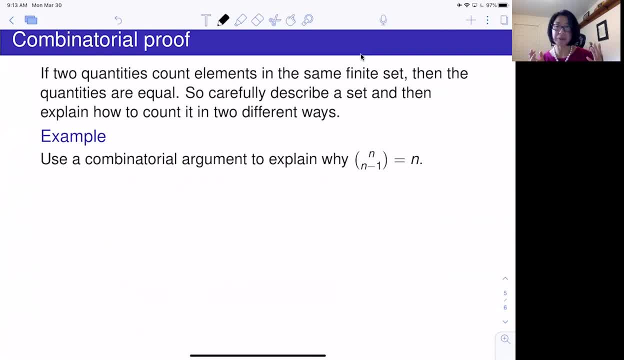 And so if two? the principle here is, you can prove two complicated formulas are the same by just showing that they count the same set, which is pretty cool. So like we can use a combinatorial argument to show why n choose n minus one is equal to n. 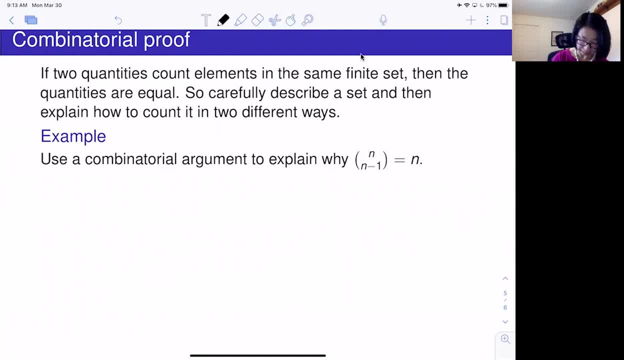 So without that formula with factorials, why so? let x equal a set with n. If x is a set with n elements, then n, choose n minus one, counts the number of n element subsets. But we can also pick n minus one element subsets. 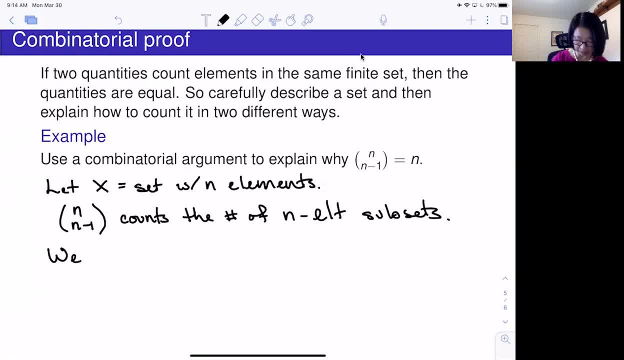 by choosing which one element to leave out, So we can also count the n minus one element subsets. Oops, this should be n minus one element subsets. Instead of sort of positively picking the n minus one elements to take, we can negatively choose the one element. 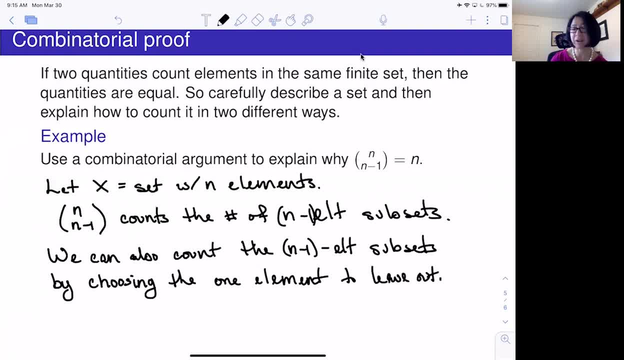 to leave, So I can leave out. and there are n elements in the set and I can leave any of them out. There there are n elements to choose to leave out. What else can we use a combinatorial proof for? So this is my favorite one. 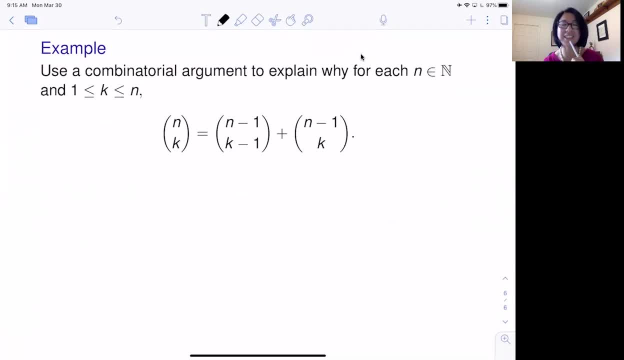 Y is n. choose k. the same as n minus one. choose k. minus one. plus n minus one, choose k. Well, here's a proof. So let's think, Suppose x is equal to a set of students in our class and we want to count subsets of k of them. 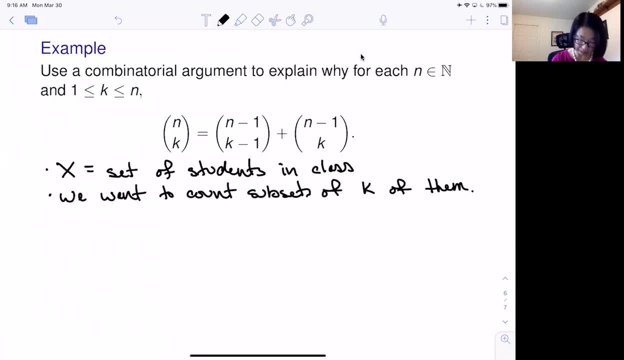 So what we're gonna do is we're gonna designate one special student. Suppose one student has a set of students. This is a purple hat and we'll call this student student p. Okay, well, so then I can say there are two cases. 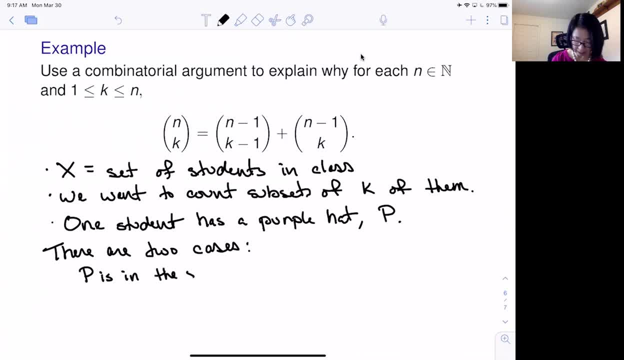 p is in this k element set or p is not in this set. So I can say there are two cases: p is in this k element set. Well, how many ways can I put choose a set of k that has the purple tatted student in it?